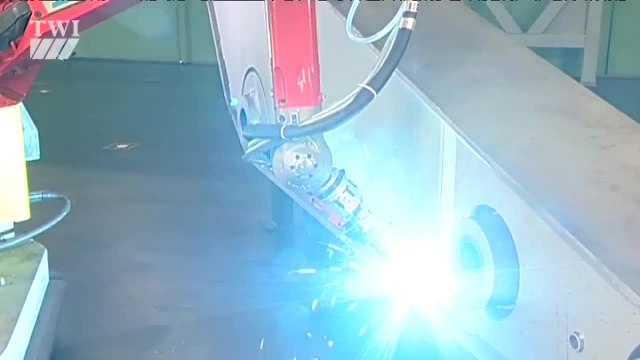 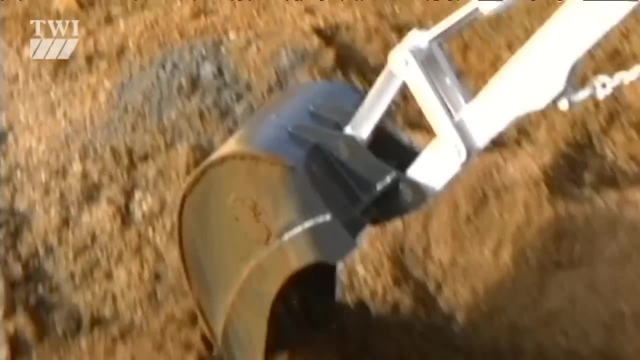 and they're also known as fatigue cracks. Excavator components are largely welded. foundry Parts are tacked together, then fully welded using MIG or submerged arc welding. In service they're subjected to a heavy load every time the bucket digs into the ground which, as 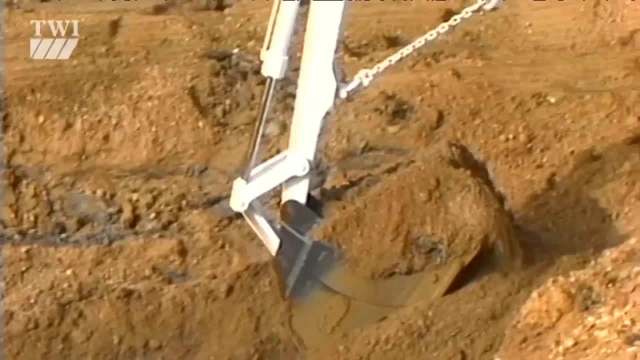 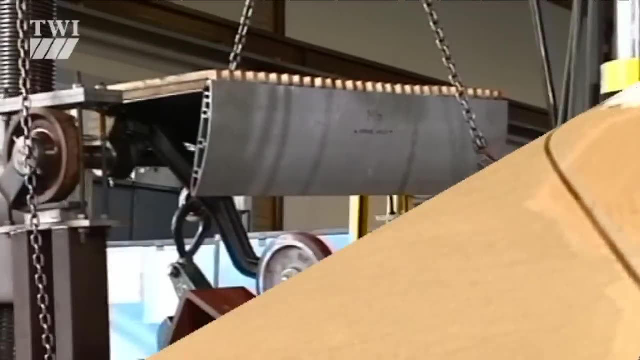 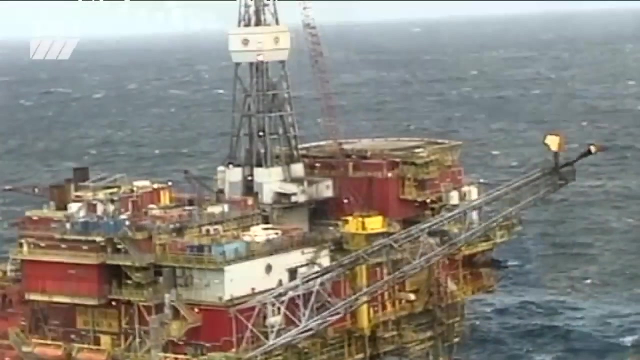 we see is pretty frequently. So the component's design, welding and inspection must reflect this fatigue loading. Small portable parts can be tested in the severest condition and the most effective is to use a fixed load. But if the job is large and in full-time service, like a bridge, support a pipeline. 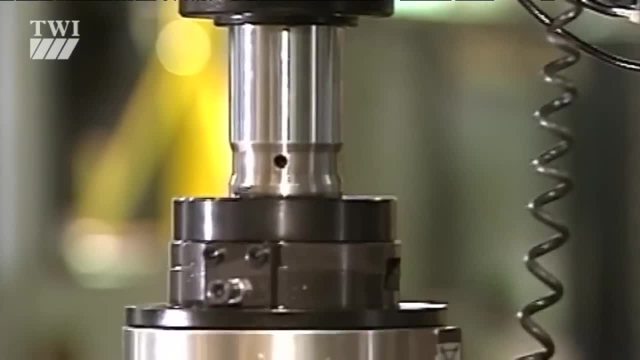 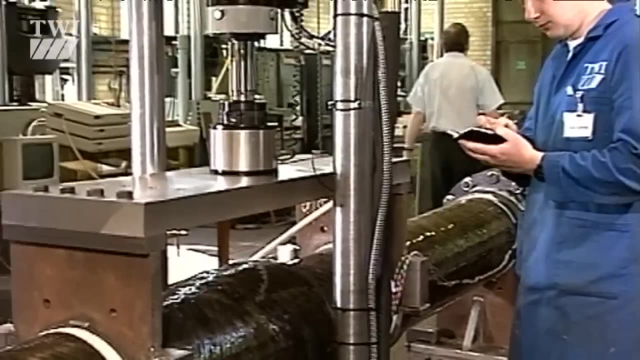 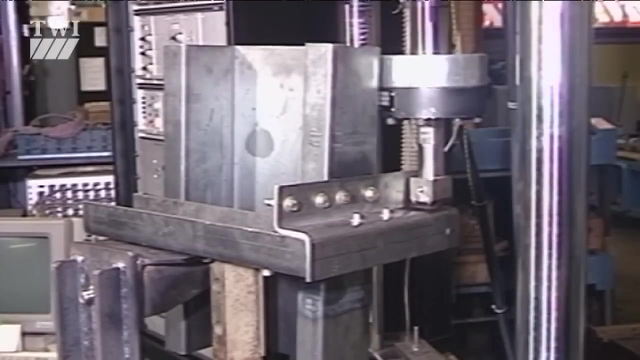 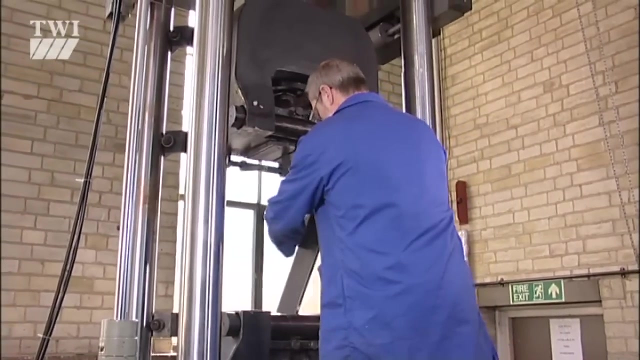 or an aircraft wing, then that's impossible. We need information at the design stage to predict the likely fatigue, wear and corrosion behaviour of the structure, And we can gather this by laboratory tests of individual welded joints. Here we use a flat plate in simple tension with attachments on either side, The longitudinal 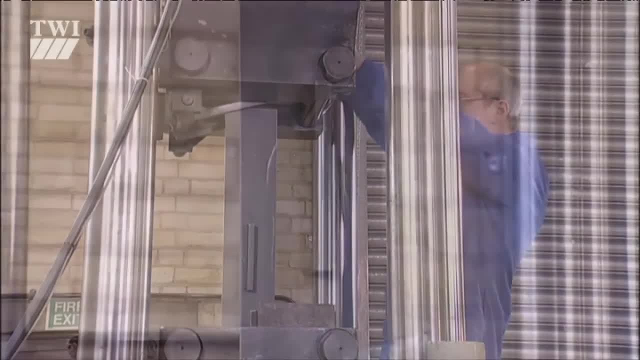 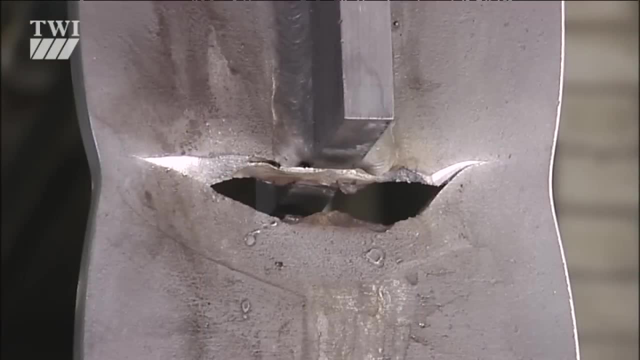 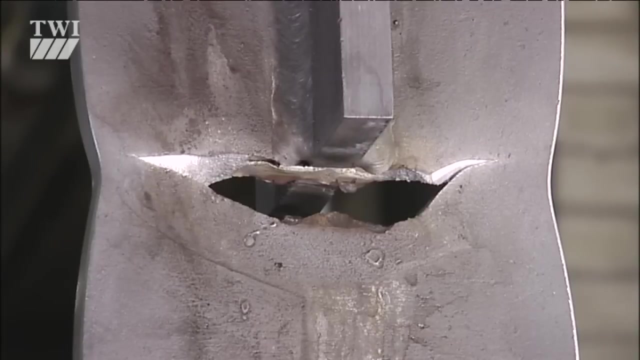 fillet welds contribute little, But we'll see, they pose a significant threat to the fatigue life of the specimen. But first a simple tensile test. Elastic deformation is followed by plastic deformation, Necking becomes evident and ductile rupture occurs. 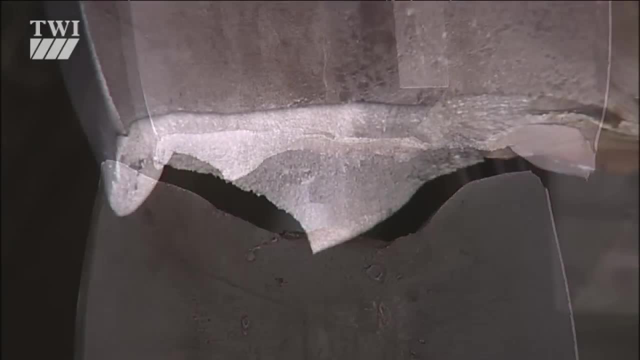 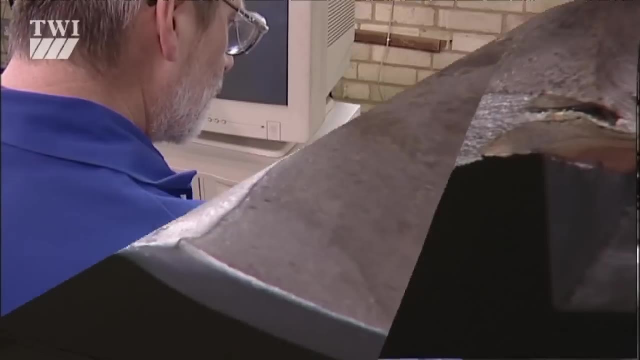 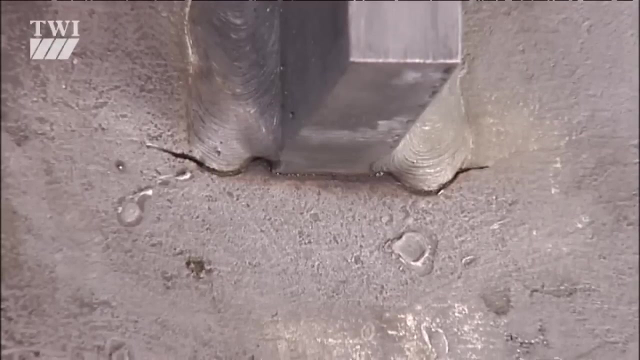 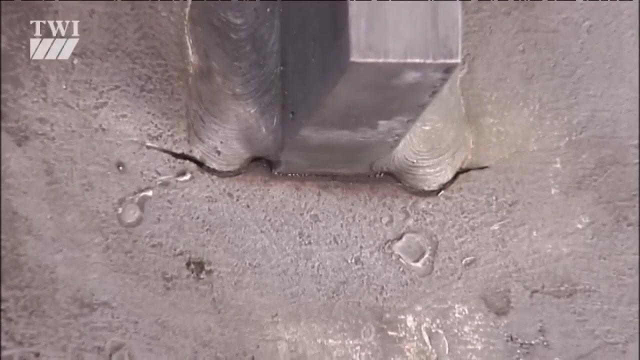 At a load corresponding to the material's tensile strength, it leaves a characteristically irregular fracture surface. Now contrast this with a similar specimen in a fatigue test. A cyclic tensile stress is applied hydraulically. Eventually it causes fatigue cracking, just here at the end of. 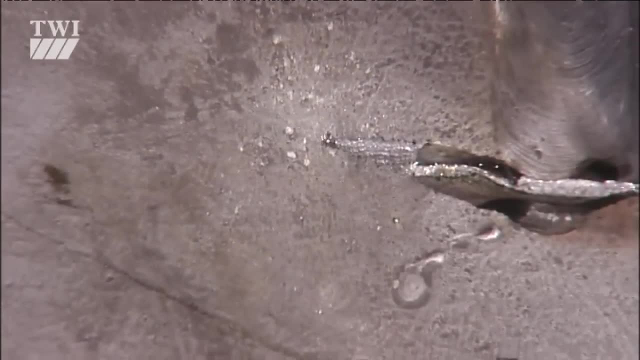 the weld. But the crucial thing is that the tensile strength is applied hydraulically. The tensile strength is applied hydraulically. Eventually it causes fatigue cracking just here at the end of the weld, And we can clearly see that this has happened at a stress well below the elastic limit. 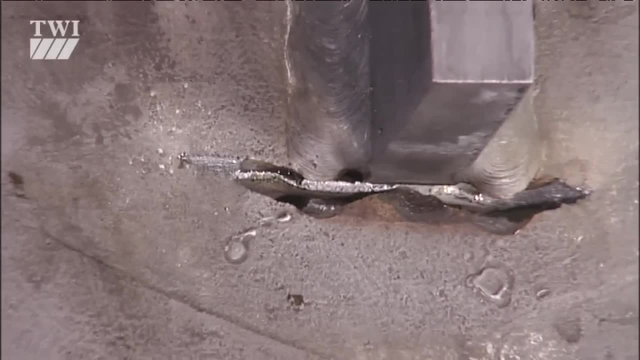 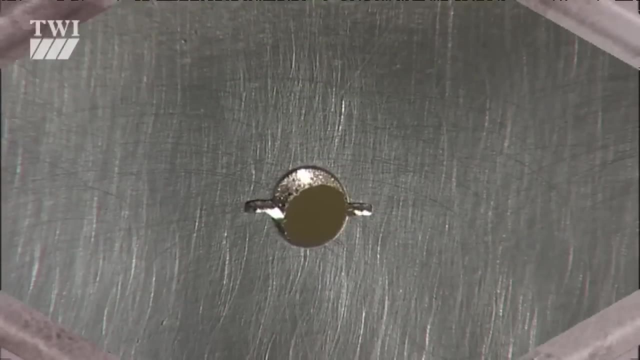 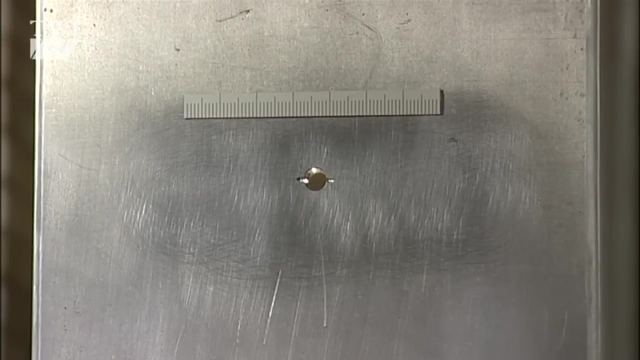 Here. fatigue cracking appears at the weld toe because of the local stress concentrations And also small weld imperfections. We can clearly watch a fatigue crack growing by testing this aluminium plate specimen in a fatigue test machine. By compressing time we can speed up the view of crack growth. 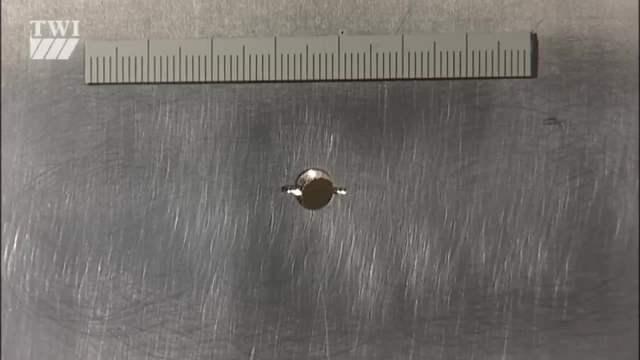 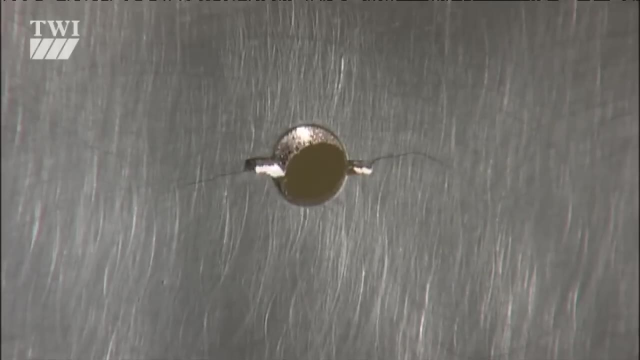 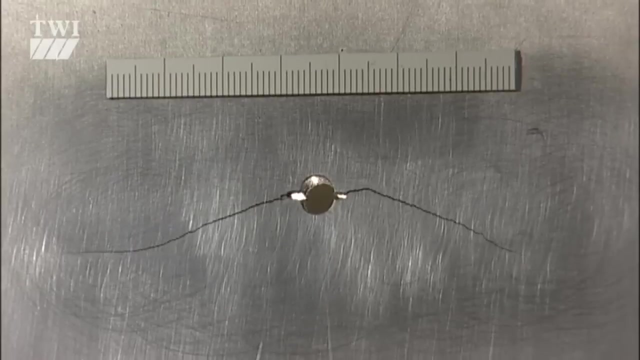 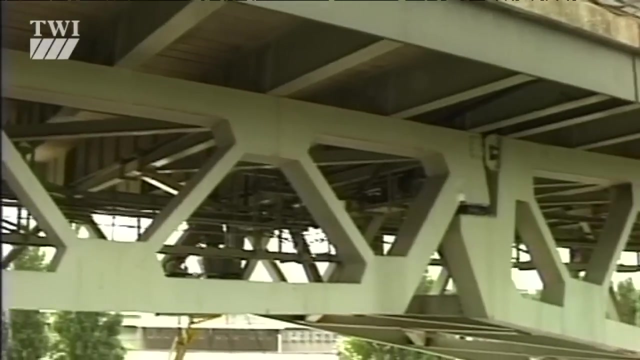 The test piece has an artificial stress concentration so that the crack is located accurately. By polishing the surface we can see the crack propagate first 10 millimetres, then 30 millimetres, to final failure. So in service it's important to inspect for evidence of fatigue early in a structure's 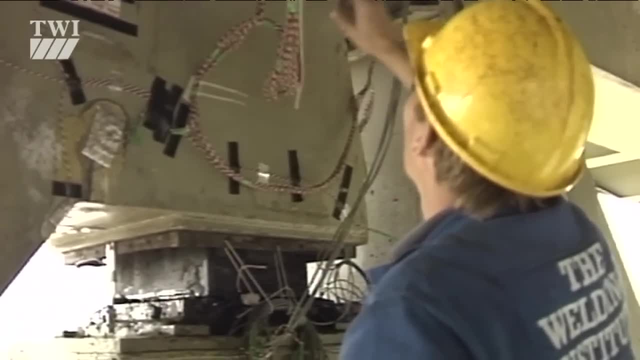 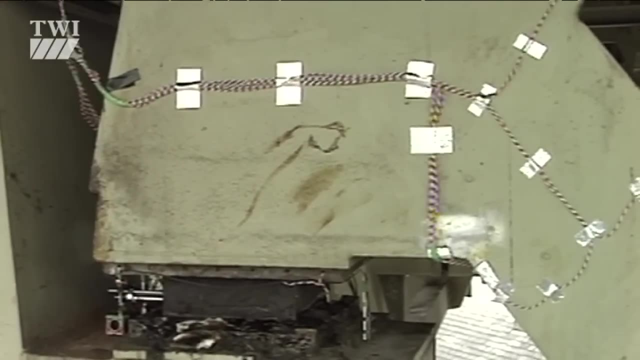 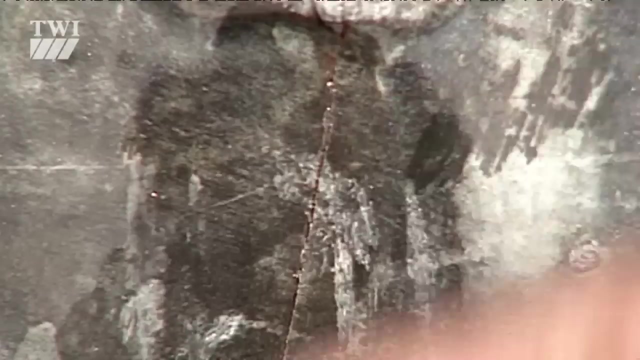 life close to load-carrying members, where the cross-section changes abruptly. Of course, rust, dirt or paint can make this site job a tough and onerous one. If it's not spotted, a crack will grow progressively until the remaining cross-section can no longer. 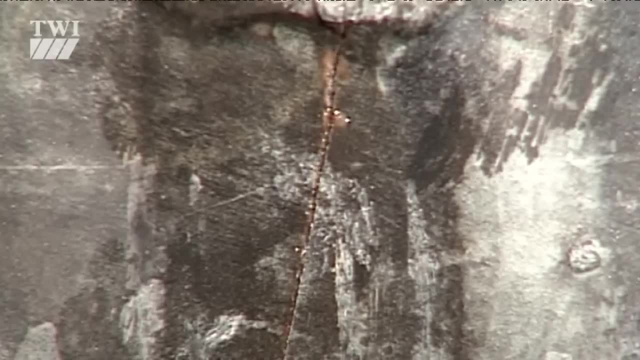 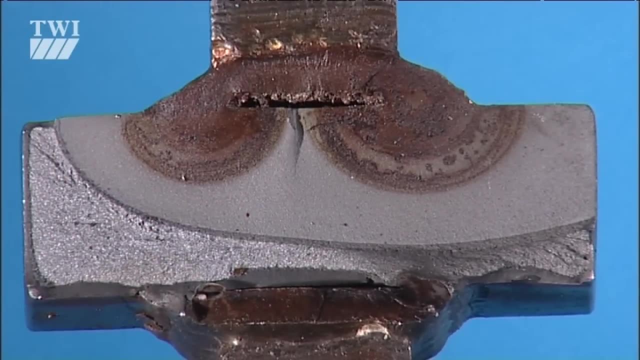 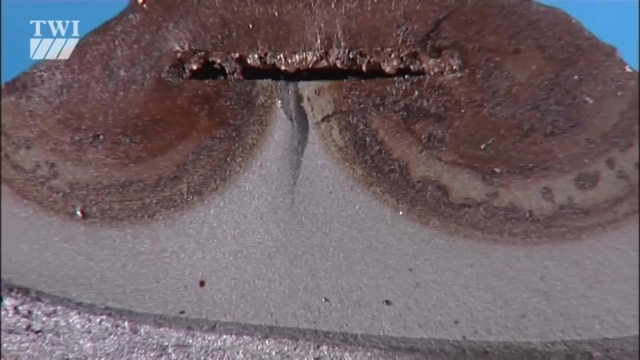 support the force applied and rapid ductile or bristle fracture occur. Subtitles by the Amaraorg community team. Fatigue crack surfaces have a distinct look about them, a smooth appearance around the point of initiation and well-defined steps corresponding to the last few cycles just. 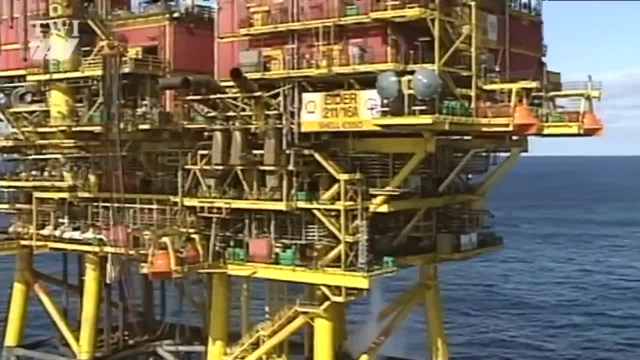 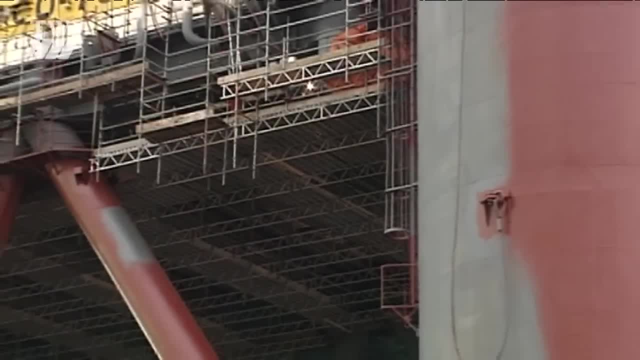 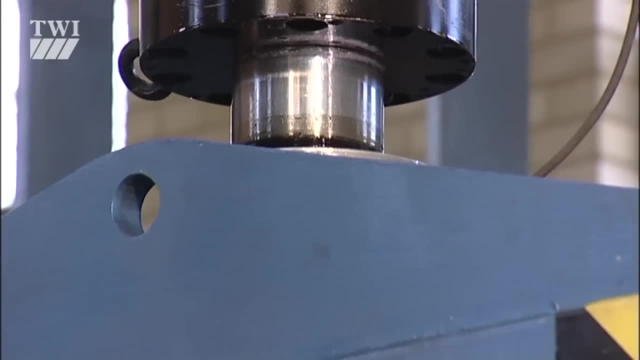 before fracture. In practice, a degree of redundancy is often present in engineered structures, so a redistribution of stress takes place and the propagation of a crack may be slowed down or reduced. There's no danger of collapse, but the structure's stiffness may have deteriorated. 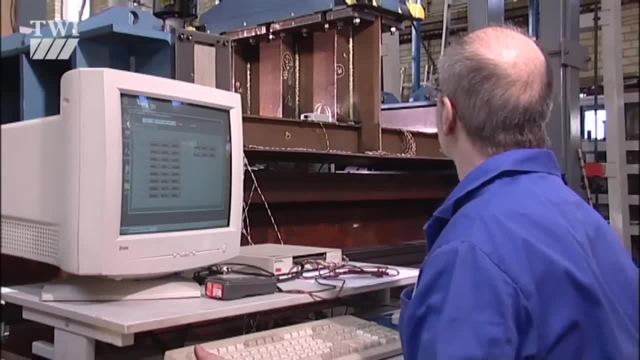 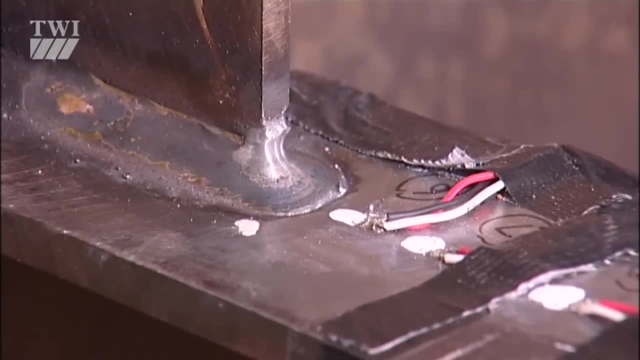 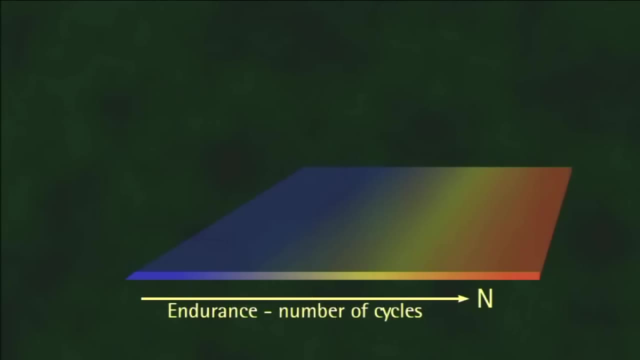 to an unacceptable level. What tests like this do is give a quantitative result of how many cycles produce a sizeable crack. So we can now represent this graphically: Numbers of cycles n horizontally And applied stress range s vertically. 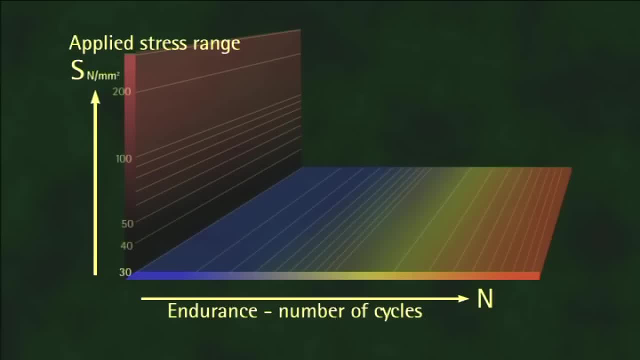 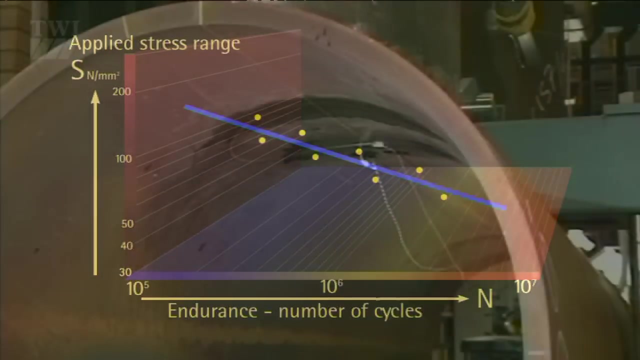 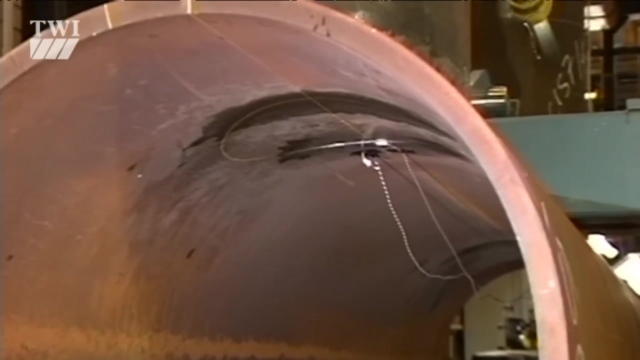 Log-log scales are used, with the horizontal scale up to 10 million cycles. in this case, By testing several specimens at different stress levels, we can create a mean line for fatigue performance. The required life of the joint, expressed as a number of stress cycles, can be related.